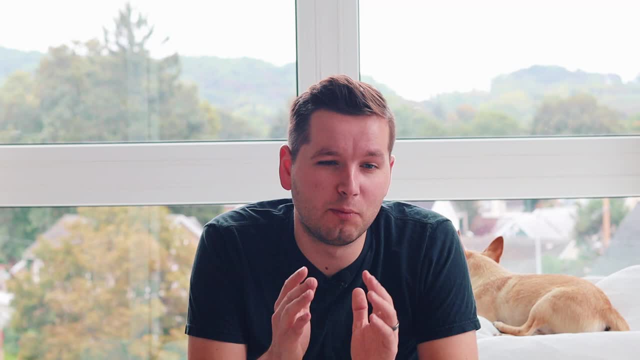 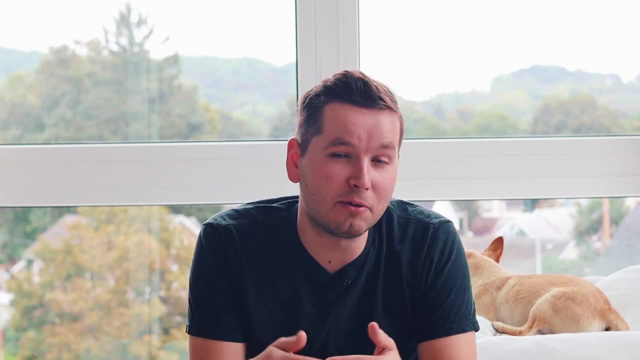 why I believe that probably 10 years from now, there won't be need to know so much about the hardware as we need to know today as an embedded developer. And even today we don't need to know so much about the hardware as the embedded software engineers, like 10-20 years ago. 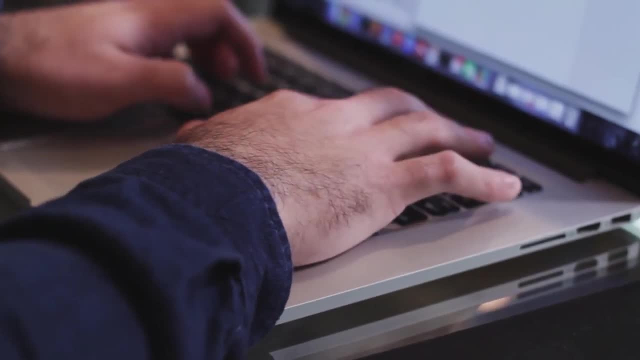 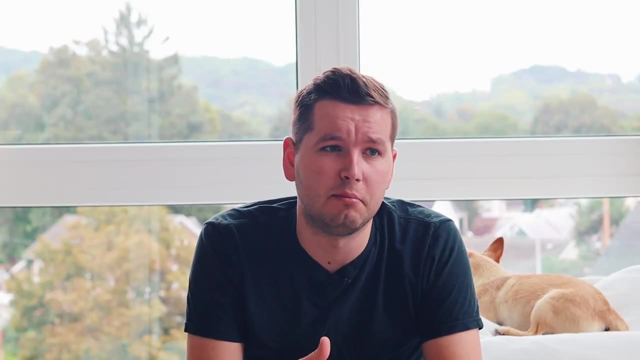 had to know. I think that the process is just getting more streamlined, so it would be easier to do the development and make it more maintainable, more generalized, make it easier for people to learn and access. Level of care is within tools used. 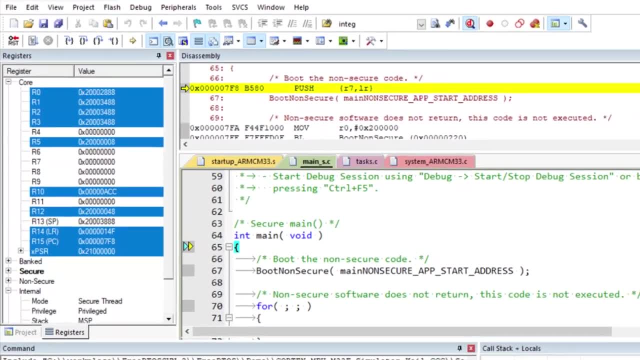 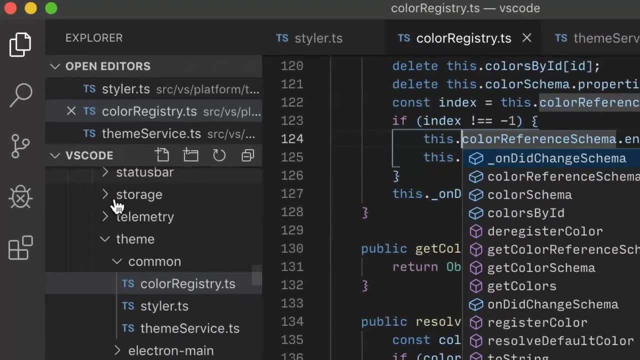 Embedded tools are often outdated and might make you feel like you're going back in time 20 years. At least, that's how I feel sometimes. General software engineering tools are typically latest and greatest. They run nice, they look nice and everyone is happy. This is why I only use 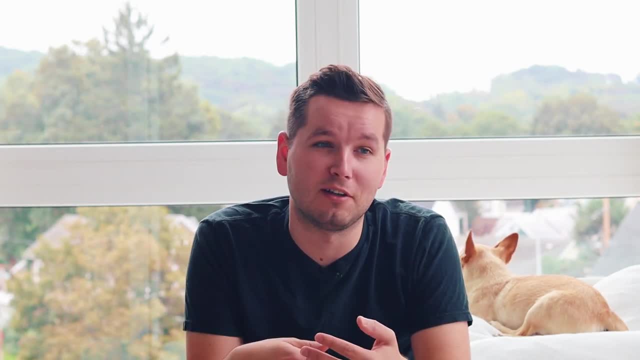 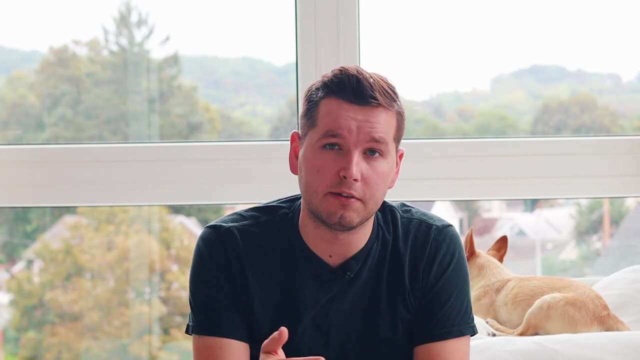 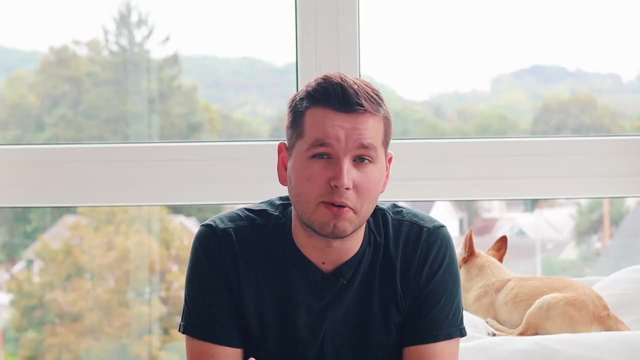 embedded tools for compiling and debugging. Rest of the work is done using Microsoft Visual Studio Code. Safety Embedded Software Engineers can often work with systems and devices where safety is a huge concern, like brake systems for cars, planes or trains, or medical devices or anything like. 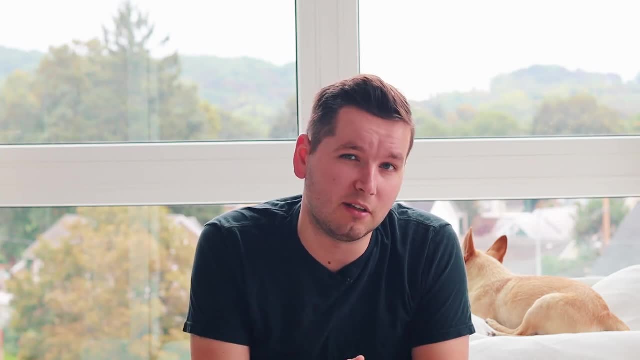 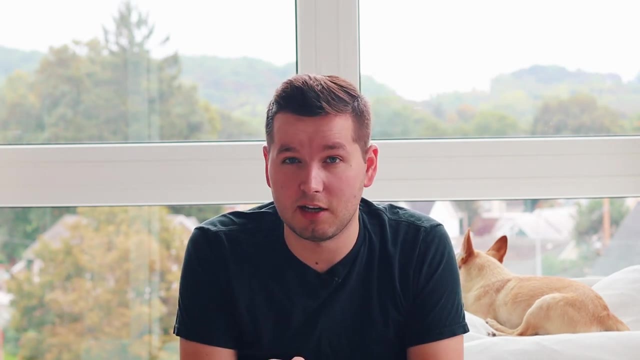 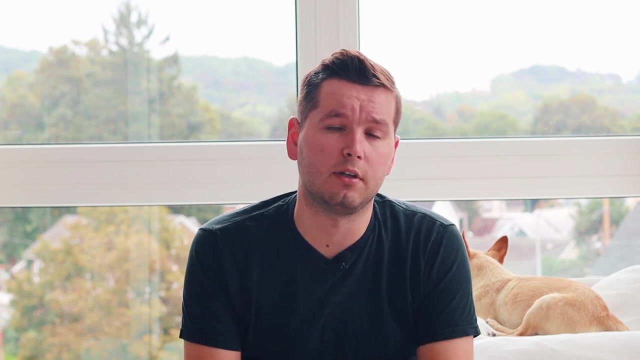 that that might result in harming a human being in some way or anyone else getting harmed Because of this. these systems can have very tight real-time timing constraints. This is not the case for regular software engineers. Yes, you might have cases where mistakes in a software can cause. 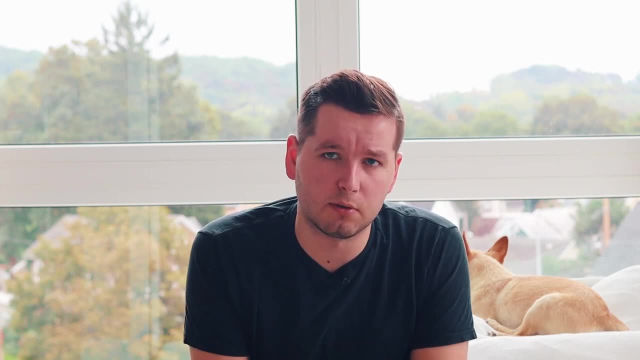 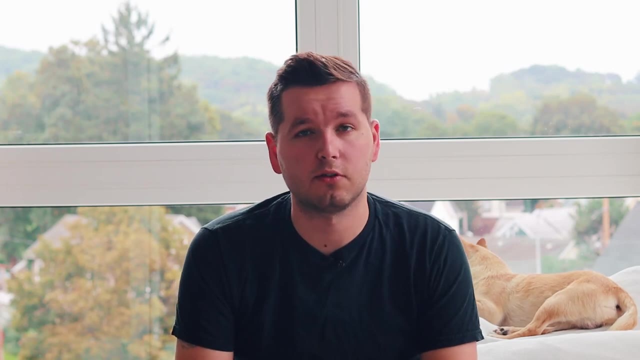 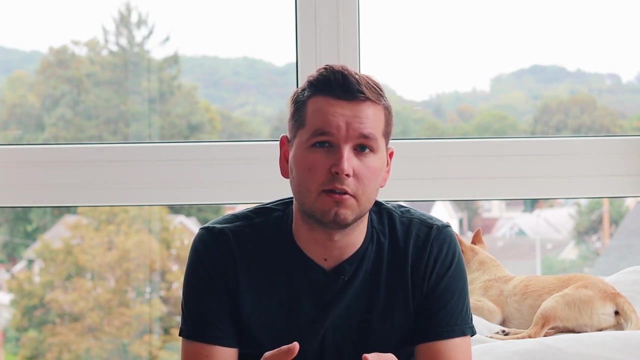 losses in your money, but typically this won't result in human beings getting hurt Resources: Embedded software engineers work with limited resources for memory, processor speed or even power consumption, Whereas when doing software development for a web or PC app, this is typically not an issue because the PCs 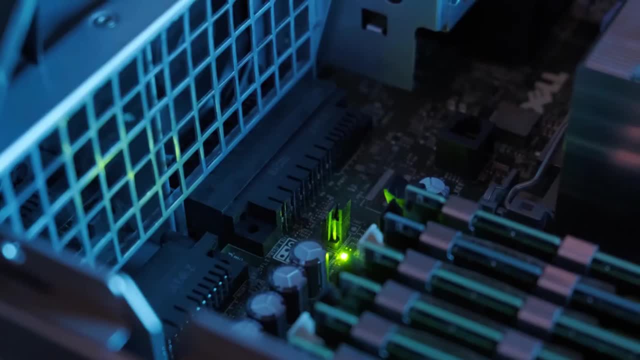 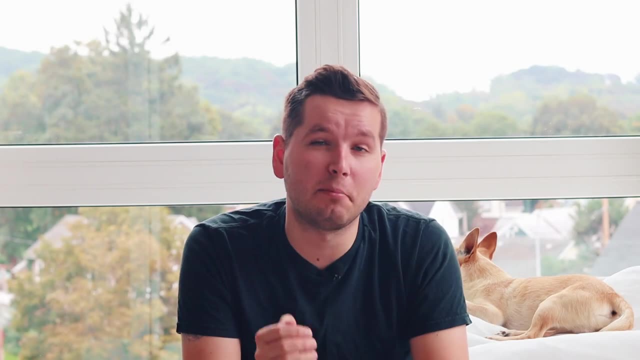 run about 20 times faster with multi-core processors and have about 2,000 times more memory and unlimited amount of power. Debugging software can be a pain in the butt for embedded software engineers, but they can also do a lot of work for other services like software. 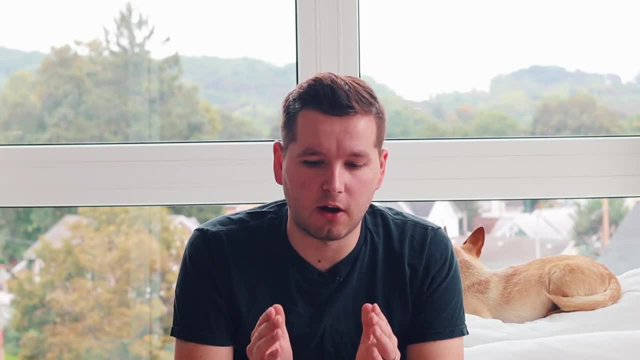 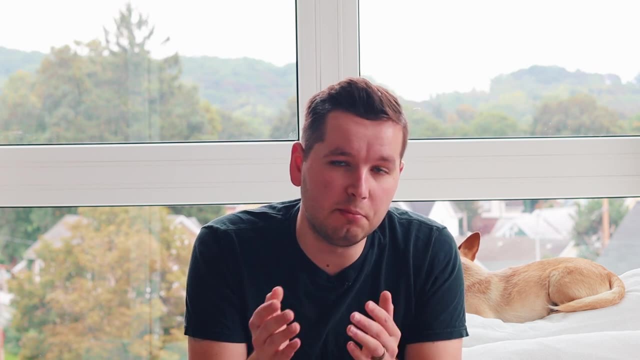 at software engineering. the reason for this is because the systems are in real time. so if you're debugging for something and you're looking for it and you stop the debugger, you might miss that issue that you were looking for. so there are some tools like logic analyzers and oscilloscope that might